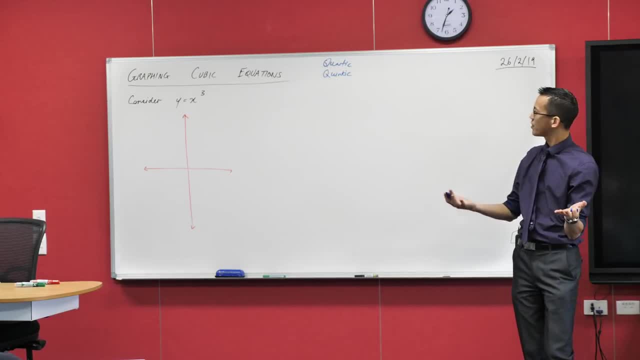 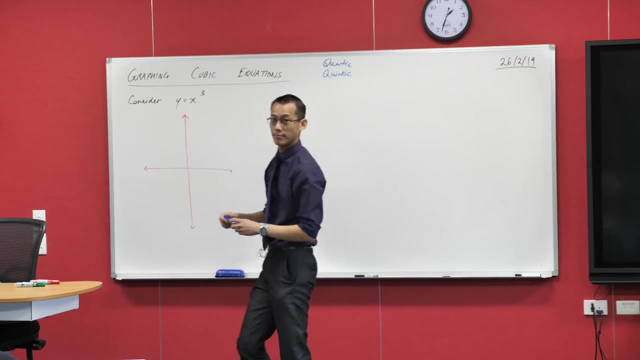 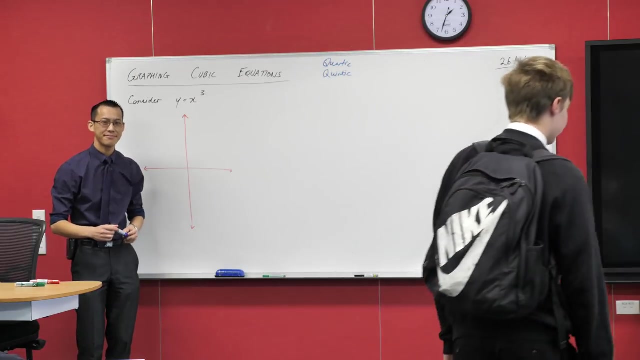 honest, I don't know if one's like Latin and one's Greek pentagon, because you don't have quintagons anyway. These continue going up, and up and up. We'll get to the circles a little later on, But all of these, all of these are in the family of objects called polynomials, right? So? 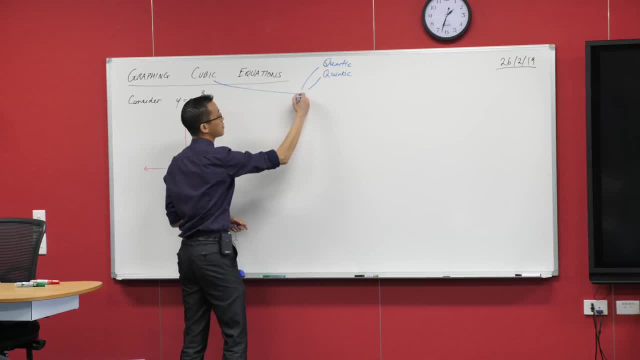 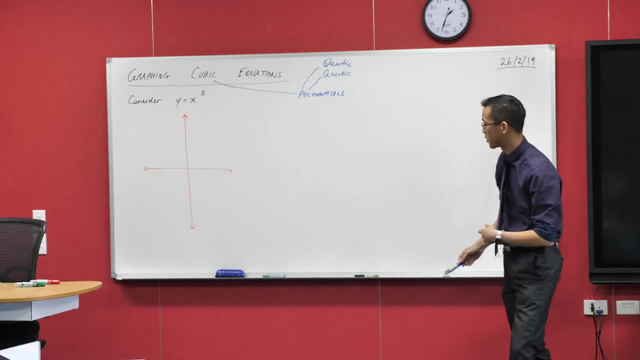 these are all, all of these guys, Okay, And, as a consequence, you have a lot of similar qualities between these. Here's the first thing I'm going to start with. You know, when you graph a function of any kind, one of the most 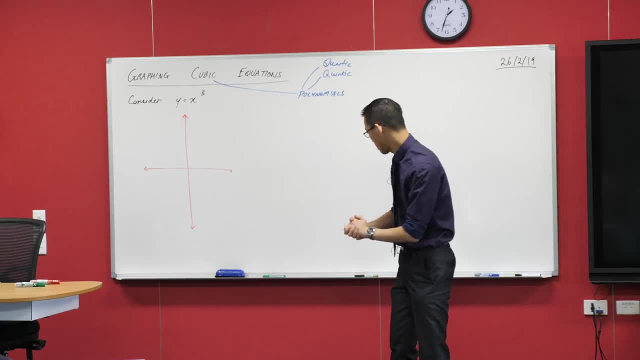 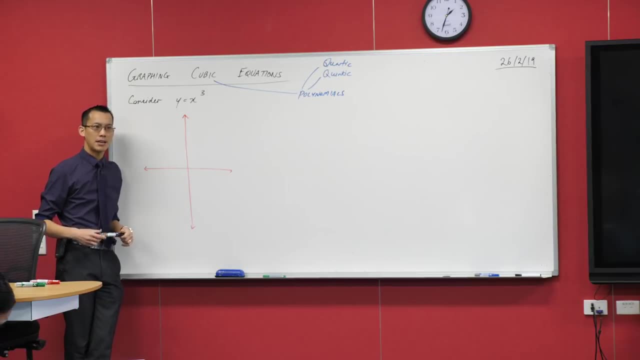 important features you're going to put on here are the intercepts. right, The intercepts. So I want you to have a think with me How much you get an intercept, any kind of intercept, out of this. How do you usually find something like, say, a y-intercept. What do you do? You let x equal zero. 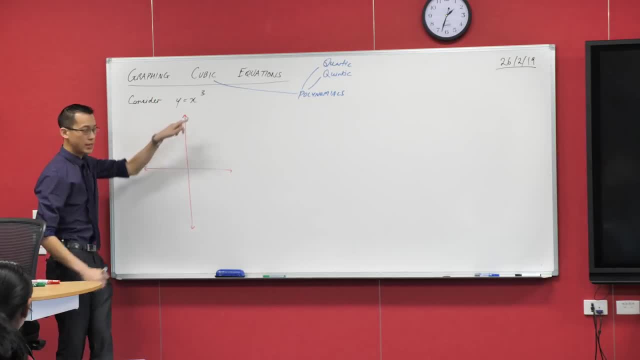 and then you'll get y equals something else, right? So if I put x equals zero into this, when x equals zero, right? By the way, really, really minor thing I'm going to say, I'm going to suggest, I'm going to encourage you to write this working that I'm about to put down here. 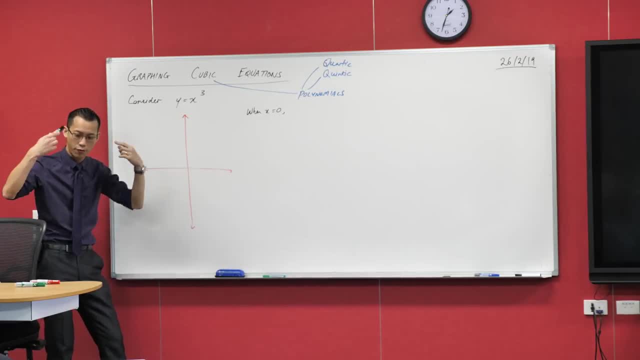 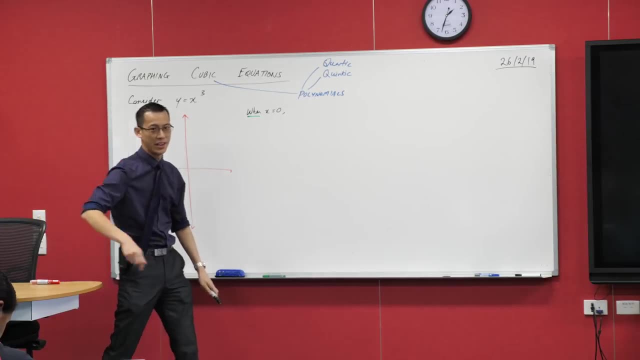 alongside your graph here because it's going to help inform your thoughts And it might seem like a little thing, but I encourage you to write the word when You're like. why do I have to put words here: When, When? Okay, I'll explain why I'm not saying let in a minute, okay, I'm not going to. 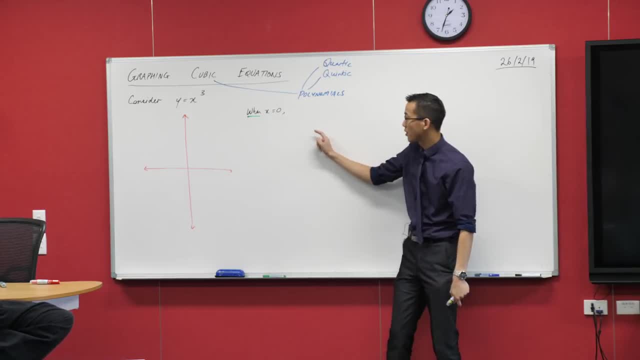 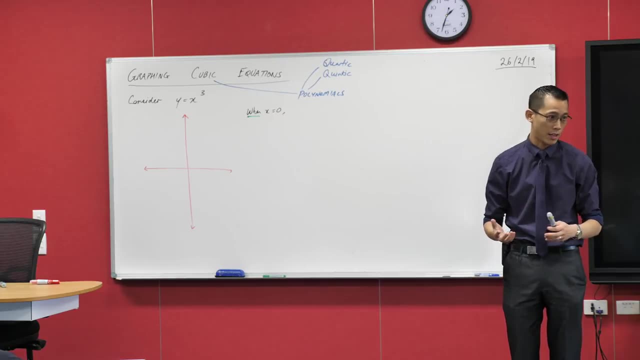 just say x equals zero and then do a thing. okay, Because the whole point behind having an equation like this is that x can be. well, let me ask you this question: What does it look like the domain? we've been thinking about domain and range before. what does it look like the domain of this function? 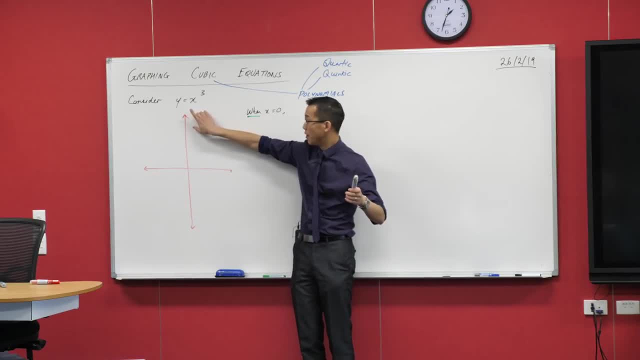 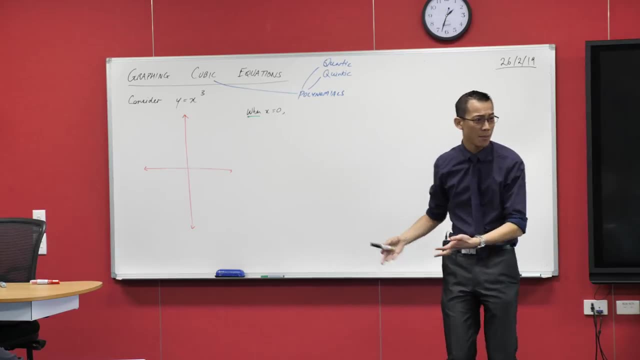 will be This: I can put pretty much any x value I like in here. It doesn't break any rules. You're never going to take the square root of a negative number. There are no square roots. You're never going to divide by zero. There's no division in here. 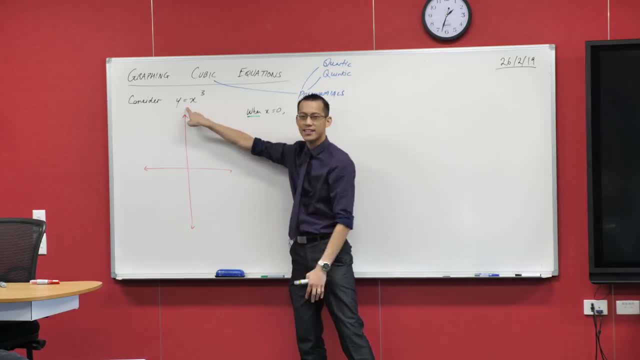 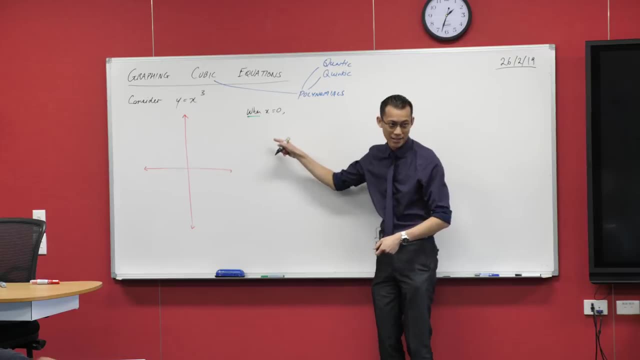 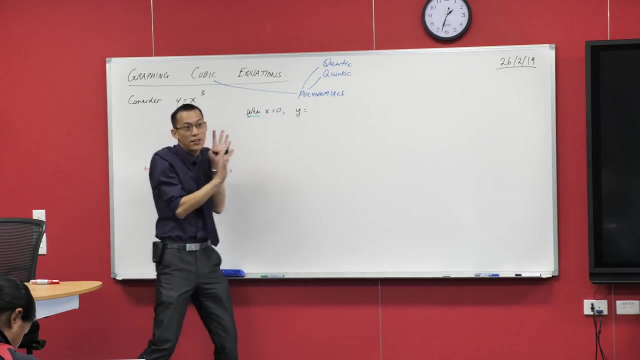 Okay, So I can put any x in here you like. And the whole point is, x can be anything, but sometimes it takes on particular values and they're going to be on our graph, right? So when x equals zero, what will y equal? I'm going to do the substitution. I'm not even going to think about it yet, I'm just. 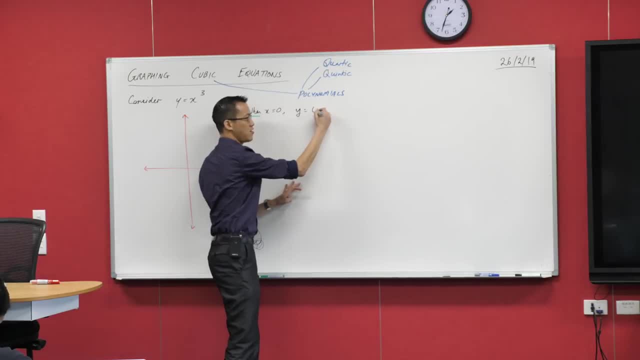 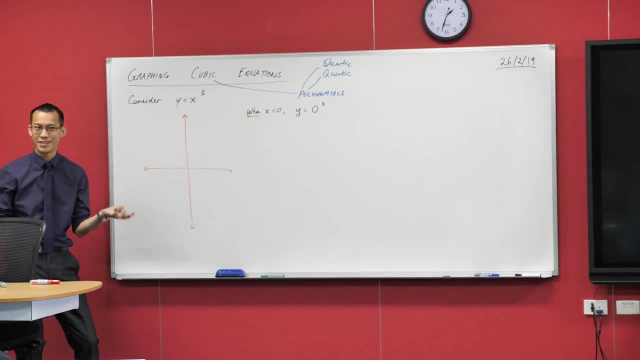 going to do the substitution, and then you can tell me what it means. I'm going to write zero instead of x- Everywhere I see x in this thing, which is only once- And then I'm going to write the rest of it. right, Zero, cubed, of course, is That's zero. 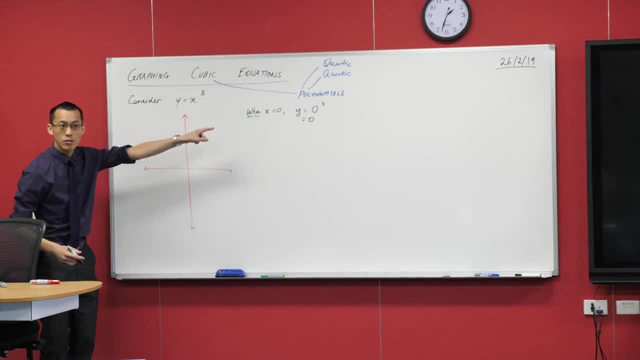 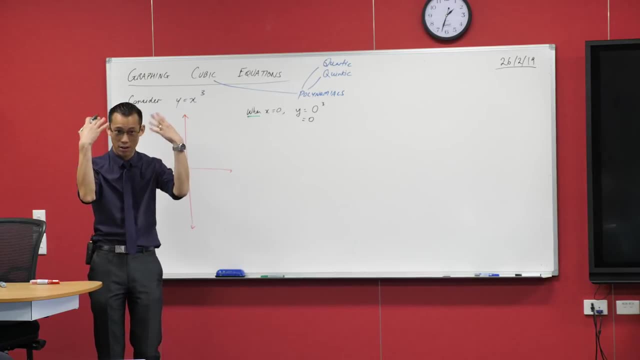 Zero times, zero times, zero. So when you see this, right, what that means is- and this part I'm going to ask you to write down. but in the future you're going to start to, you're going to stop writing this because it'll become like apparent to you, right, What I can say is, on the basis of: 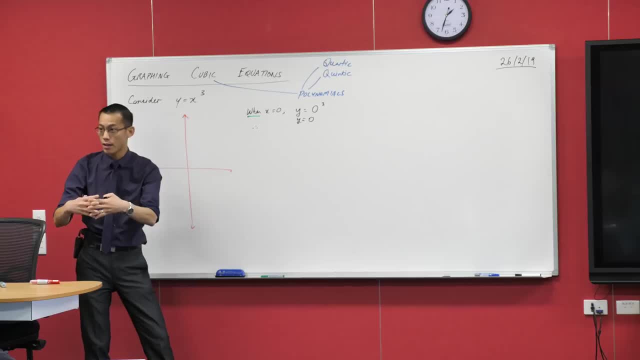 this right that I've got an x and a y together. this is a pair of coordinates, right? So what this is saying is zero, right? there's the x, there's the y is a point on my graph, right, When I do. 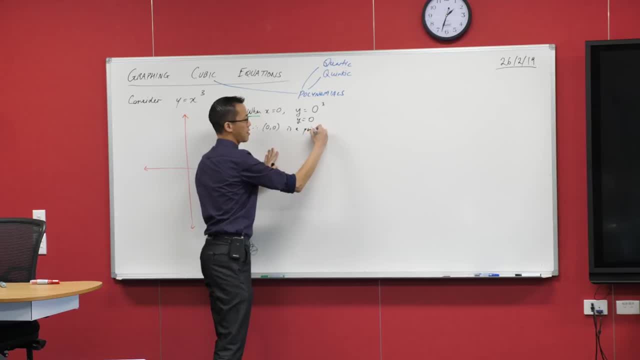 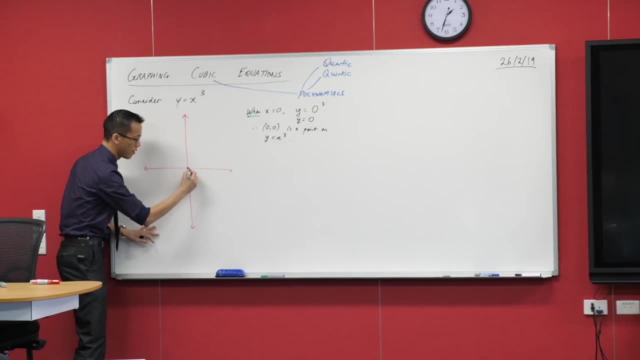 my draw right: Zero. zero is a point on y equals x cubed on my graph. okay, So I'm going to go ahead and I'm going to place that onto my set of axes, okay? Oh, by the way, I probably should have. 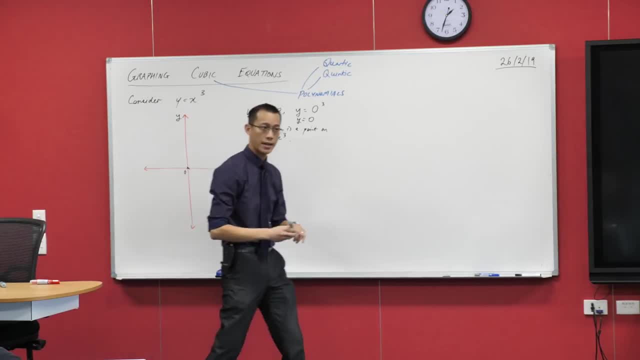 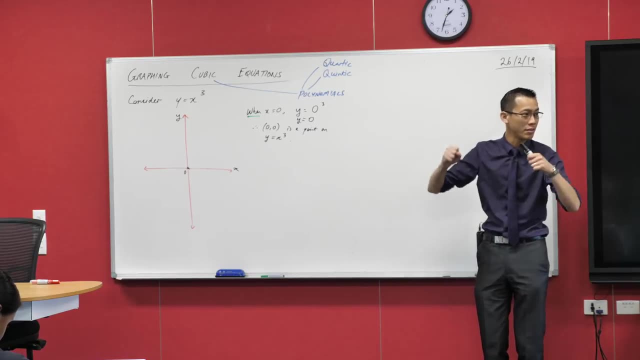 labeled those. You get the idea. okay. Now, we could keep on doing this for a while, but it looks like we've got an x-intercept and a y-intercept all in one. That's a nice bonus, okay, As I think. 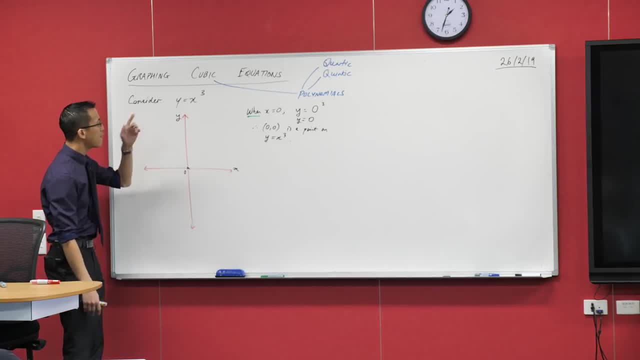 about what's going to happen. as I put in a x-intercept, I'm going to put in a y-intercept. I'm not going to write these anymore. If I were to put in one for x, what would I get? I would get. 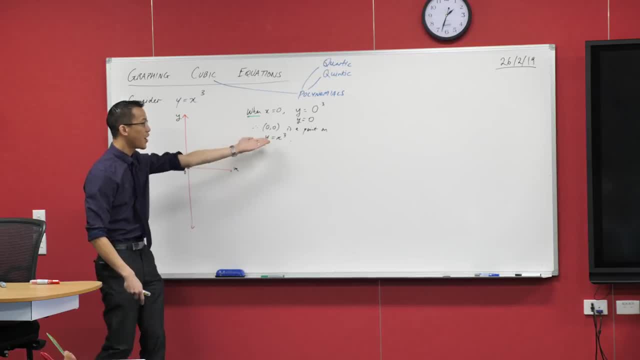 y equals one. So one comma one is another point on my graph. I'm going to place that here. One one. okay, When I put two into here, what's y going to be equal to? It's going to be eight, This thing. 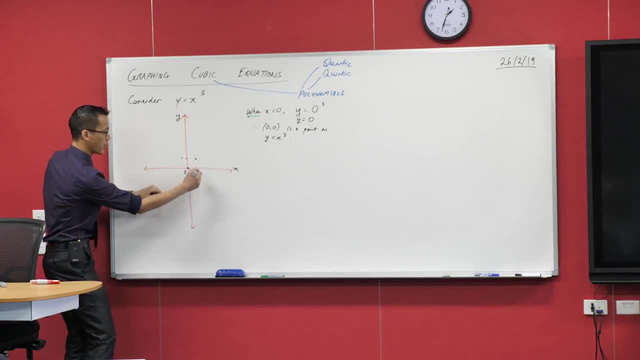 is skyrocketing and it's skyrocketing fast, right? So if I go across the two, I'm already up here at eight. Does that make sense? Two comma eight is a point on my graph, So you can see this thing is sort of ratcheting up all the. 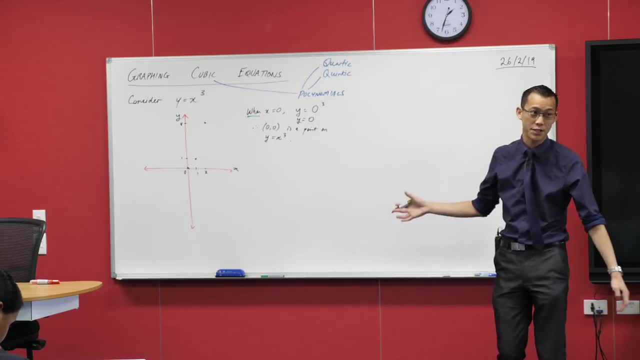 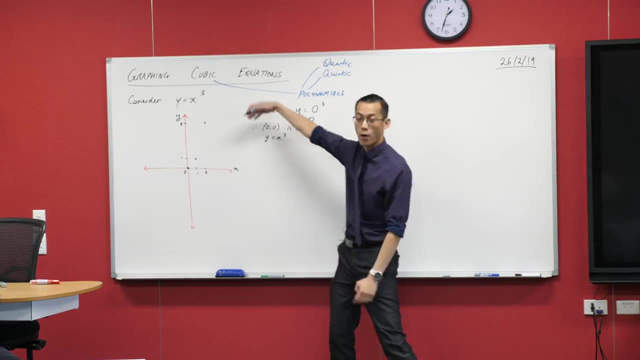 way right. It's going to climb fast. In fact, I already no longer have space on my graph anyway. to put the next thing, If x were equal to three, what would y be equal to Twenty-seven? Three cubed is twenty-seven, So that's way off my set of axes. So okay, it's going to be up the top. 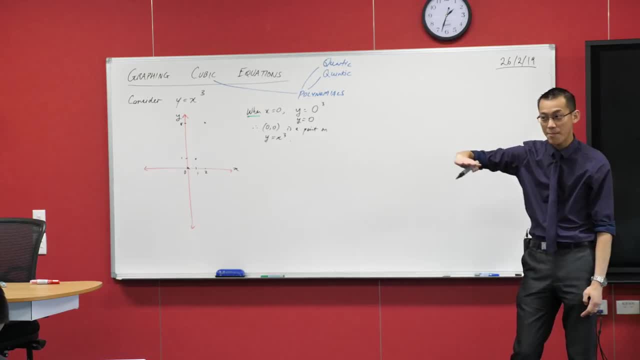 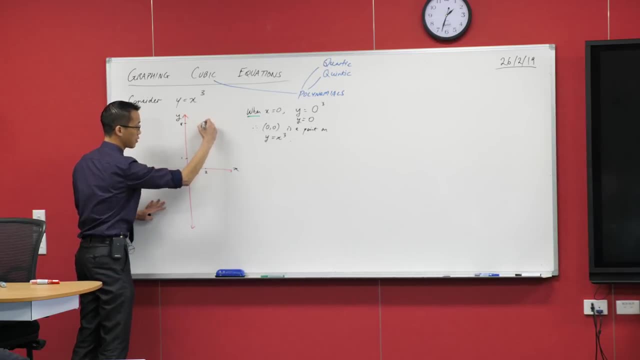 right. So that's what's happening. on the left-hand side It's getting steeper and steeper and steeper as we go. So I could actually connect up the dots sort of thing over here. I could say, oh, this is going to sort of come down like this: It starts off nice and slow and then it. 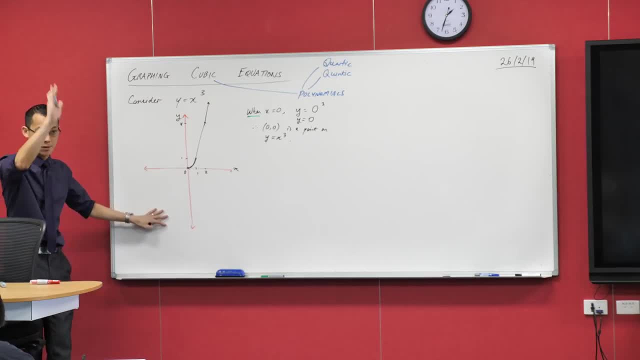 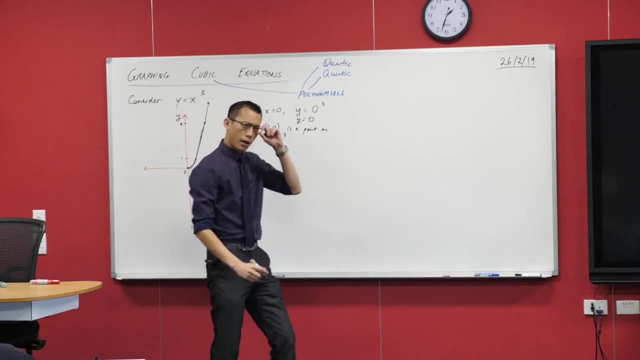 just kind of races off really, really fast up in the positive direction. okay, It's not a great graph, but I'm going to run with it still. I think it's close enough for our purposes. Okay, so I've got the positive side of this. but we established before that the domain also exists over on the. 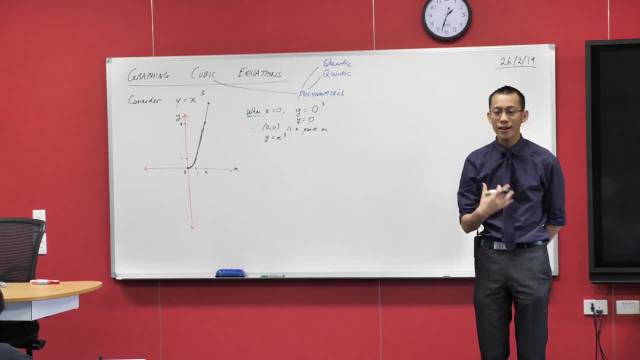 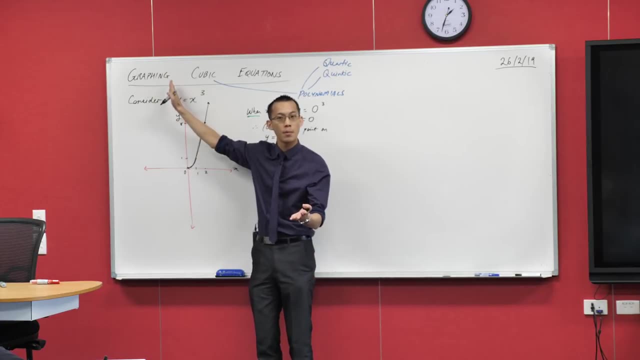 left, right. When I put negative values into here, though, unlike when we thought about the quadratics, right The quadratic, the parabola is going to go off in this direction, because when you square a number, what happens to? 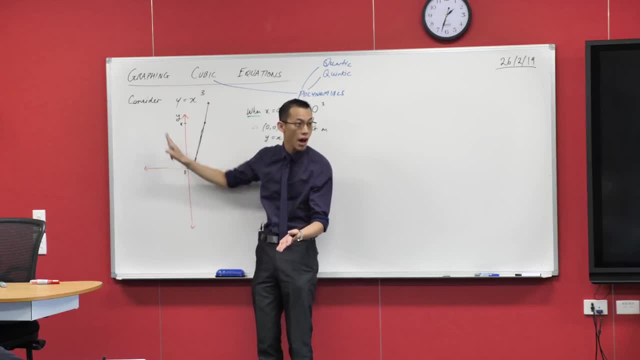 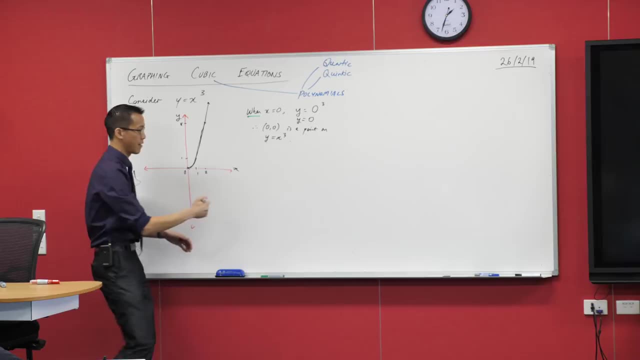 the sign. It's always going to be positive, right, So you stay up above, right. But this doesn't happen for the cubic, does it right? It goes down because if you were to put this, one is worth writing, right? If I put in, x equals negative one, right, So I can take on this value. 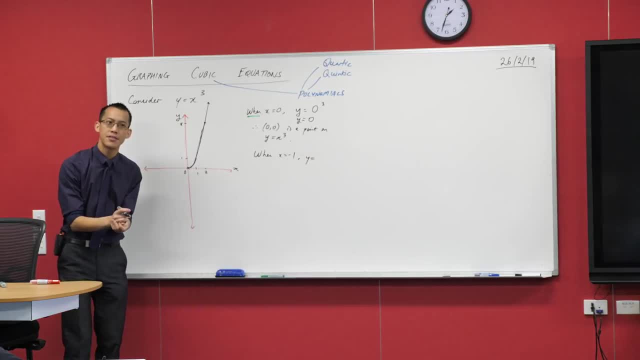 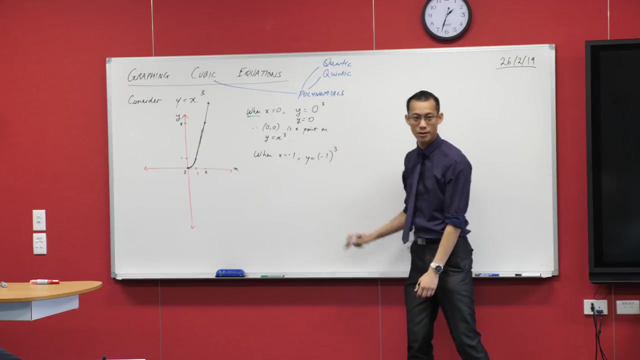 two Y is going to be equal to. just be careful how you write this, yeah, Especially when you put this into a calculator, you can get quite confused, because your calculator will tell you exactly what this is for, unless you answer it wrong. Okay, yeah, so this is negative one, cubed, as opposed to. 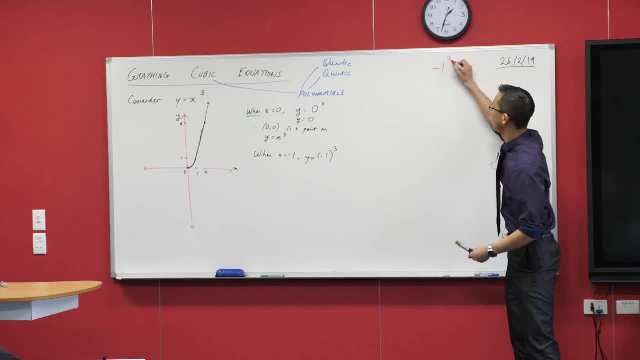 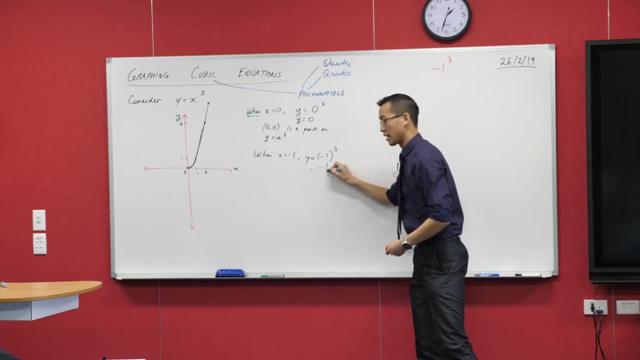 I'm going to don't write this down- as opposed to negative one cubed. right, These are two different things. It just so happens. coincidentally, at the moment they're the same. That's just negative one. but your calculator thinks about these differently. right, It's going to go negative. 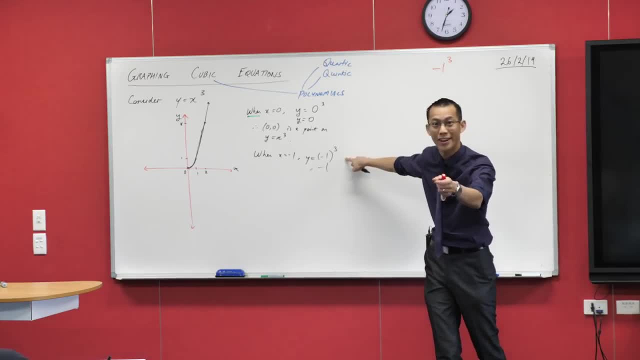 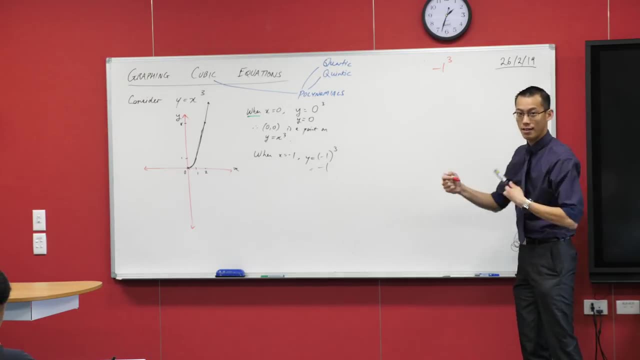 one times negative, one times negative one. Your brain should think about it differently as well, right? And if it's two, it's just one. Exactly right. If I did negative one squared. those are quite different, aren't they? Yeah, do you have your calculator there? Do you have your? 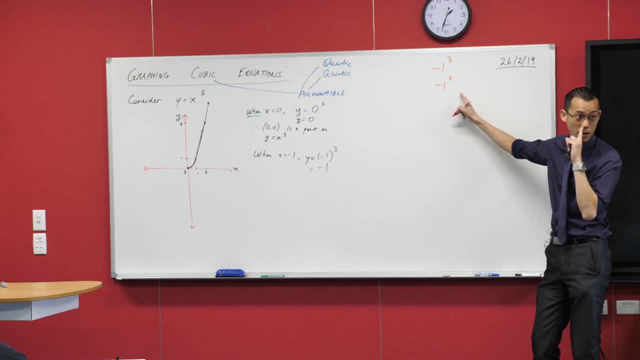 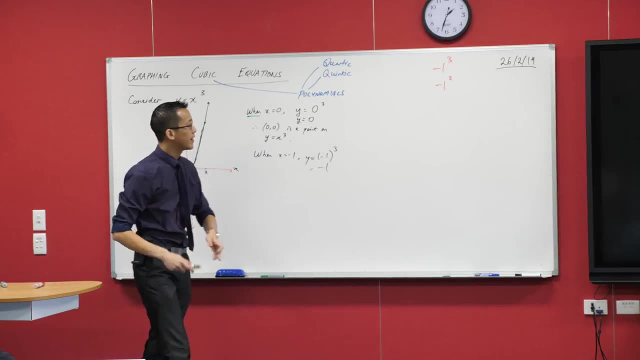 calculator there. If it's not get it out, If you pop this into your calculator, right, What's it going to do? What does it actually tell you? Yeah, no brackets. It says: oh, I know what. it has an. 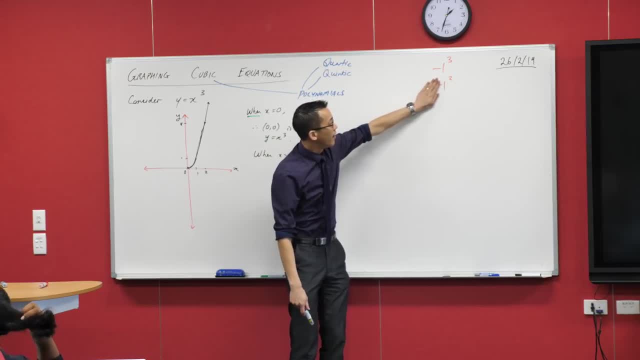 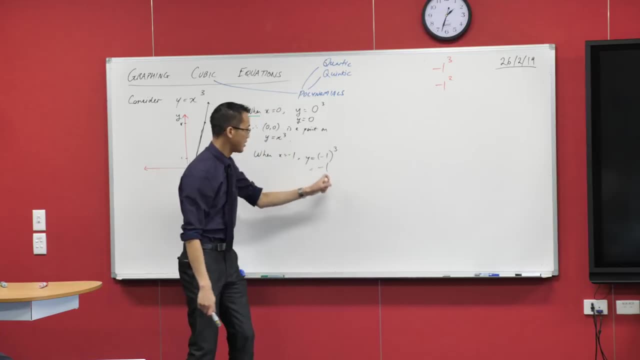 order of operations built in. Yeah, it squares the one right. And then it's like: oh, you want a negative as well? No problem, I'll give you negative one, right, But of course, negative one. if we did this, it's going to be negative. one times negative, one times negative, one right. So 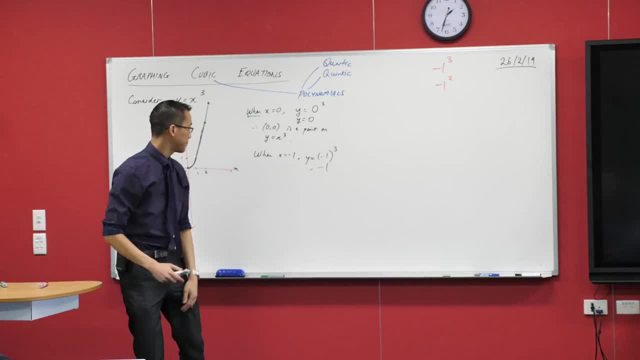 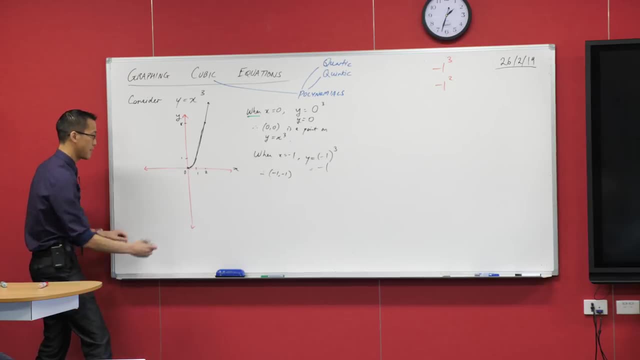 if I did this twice, it'd be negative, one times negative one. they would cancel, okay. So what does this tell us? right? I can say, therefore, negative one, negative one. that's on my graph, right? I'm going to put that there. I'm going to make sure this is consistent And you can see. 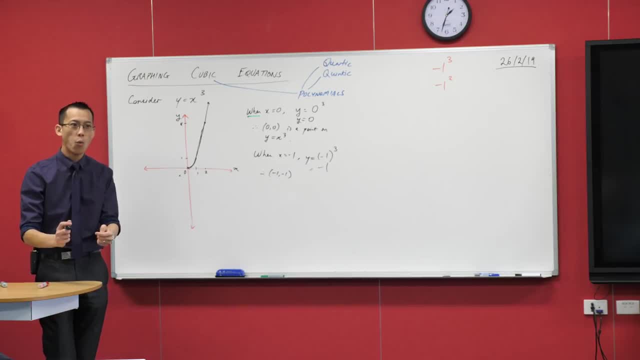 there is going to be a symmetry to this graph, right? What kind of symmetry is it? We have a name for this, don't we? It's the. it has rotational symmetry. I could spin this, this graph, I could spin it around, So it goes sort of down like this, right? What's the name of this? It's. 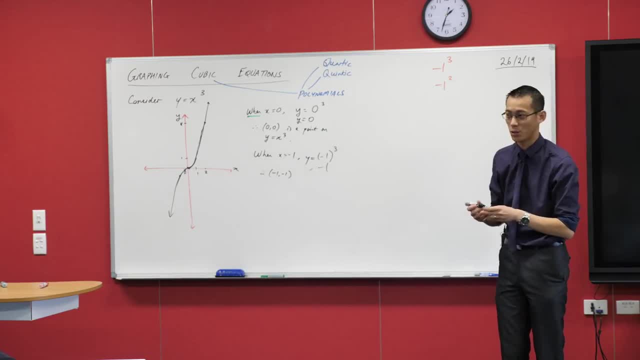 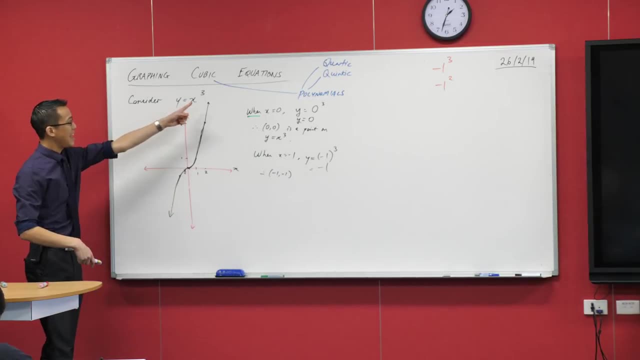 odd symmetry, isn't it? And we actually, to remind you, because I know with Mrs Liz you looked at this already- part of the way you can know why odd symmetry is called odd symmetry is: have a look at the power, right, It's an odd number And in fact, any polynomial which has this kind of structure. 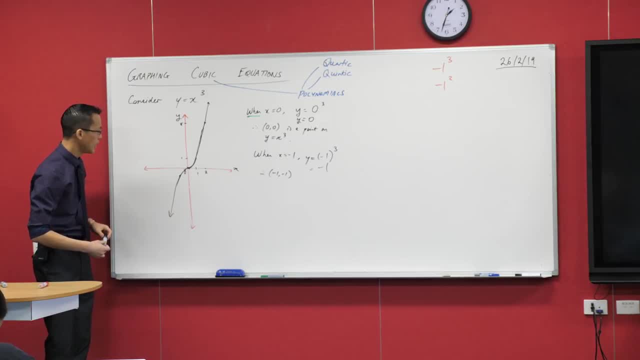 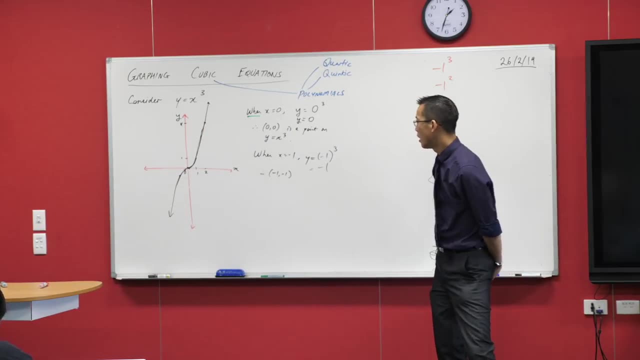 is going to have this kind of symmetry. okay, All right. Now this is more or less. y equals x. cubed, Say it again. What would be the second point? Minus two, Minus two, Minus two minus eight. 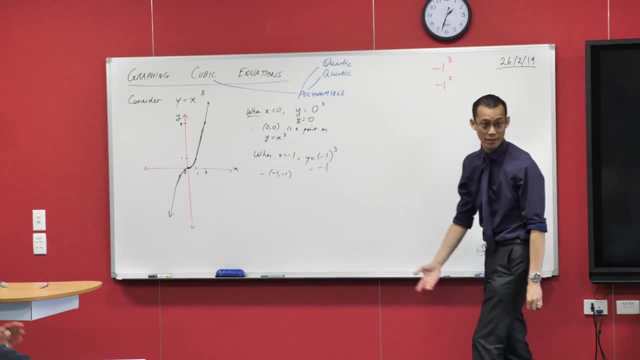 Minus eight because it's going down, isn't it Okay? And you can put more points on to get more detail if you want to. okay, Now, I'm pretty happy with this right. This is the graph of y equals x. 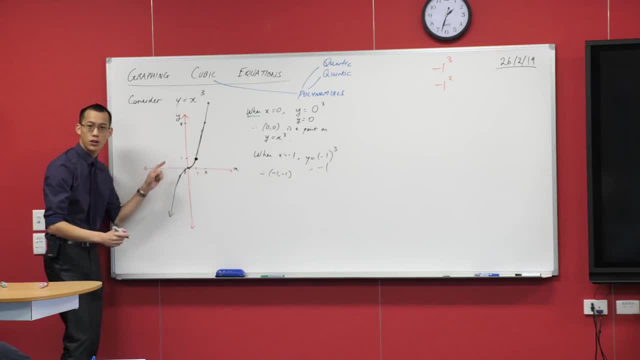 cubed, Just for the sake of it. I'm going to re-emphasize: I've got this point here right And I'm going to draw on here something that indicates exactly where it is, Because if you went to Desmos, for instance, and you put in y equals x, cubed, you'd get a shape like this: 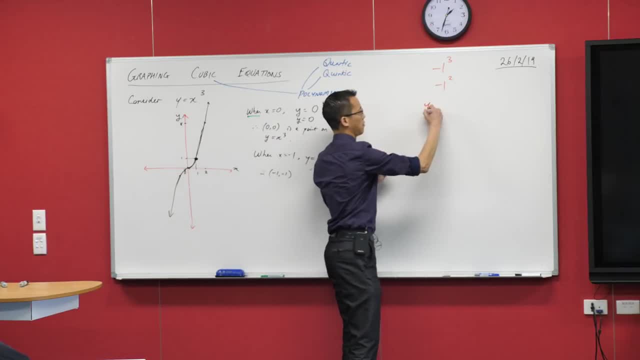 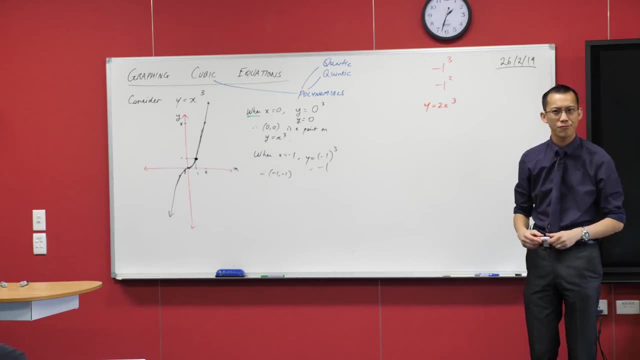 right, But if you put in something like y equals two x cubed, you'd get almost exactly the same shape. What would be the difference? by the way, It would be slightly different. It would be that way. So there's going to be some squishing and scaling, but which way, Rassan? what are you? 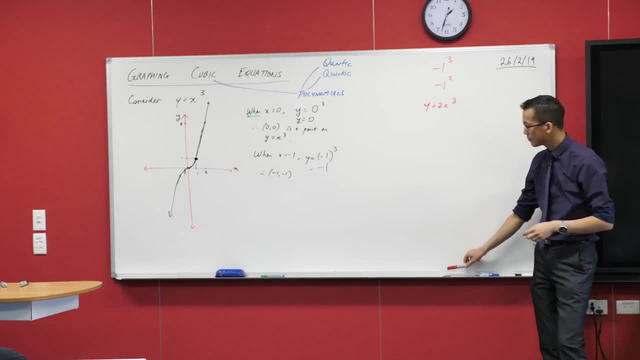 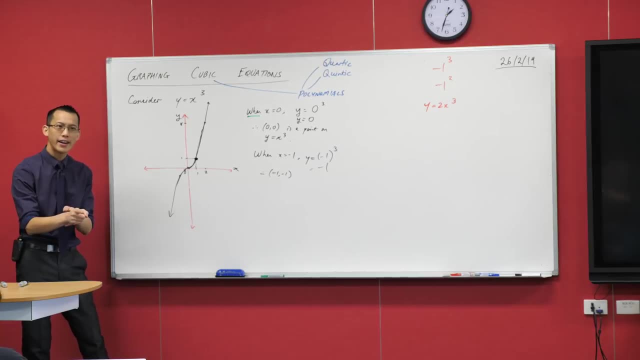 thinking: Well, since it's a two x cubed, so whatever value of x you put in is going to be two times more than equal. Exactly Right. That's really interesting. Okay now, this is not our main point. okay, It's not our. 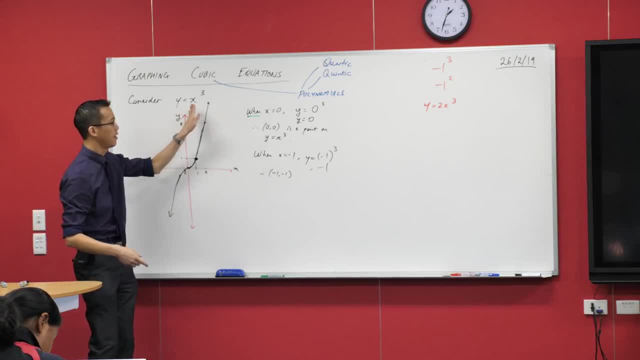 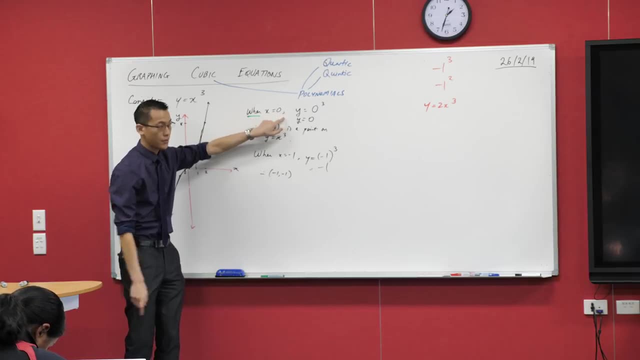 main point, but I do want to think through this with you, because you're going to be getting some of these later on. okay, If I went through this same process, right, Let's have a think about this one, right? When x equals zero for that guy over there, what would happen? 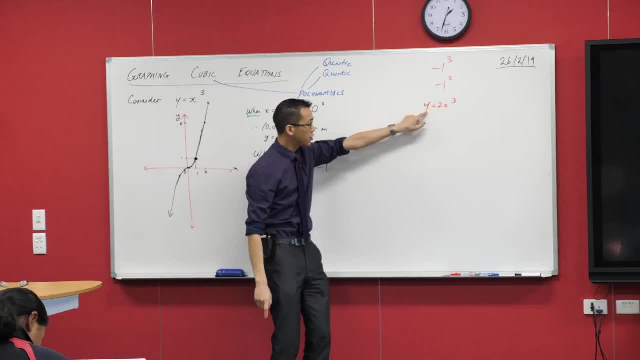 when I went through and substituted x equals zero, It'd be zero. Yeah, it's going to be two times zero, still zero. So y equals two x cubed would still go through that point there. zero, zero, Right Right. 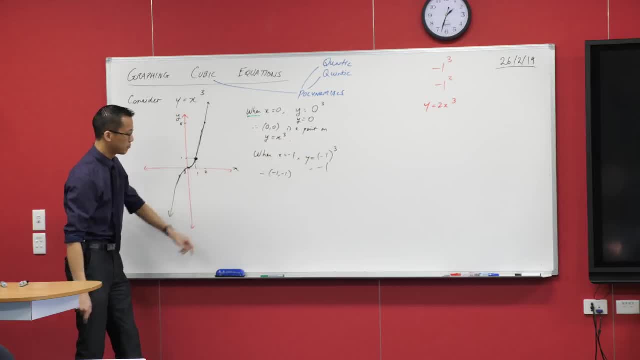 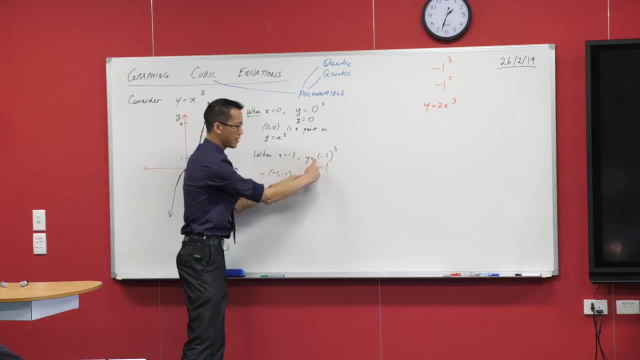 When I put in negative one. okay, this is still going to be the same, but there's going to be a two out the front, right? So what would happen on this line? Just for this particular one? that we multiply by two gives me negative two, right? So instead, 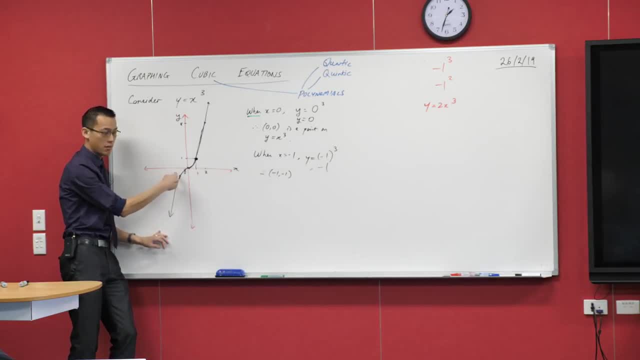 of being here at negative one, negative one. I'm going to be at negative one, and then I'm going to be twice as far down. I'm going to be down here at negative two, Do you agree? Right, Right? And instead of being at two eight, I'm going to be twice as high up. I'll be at 16,, right. 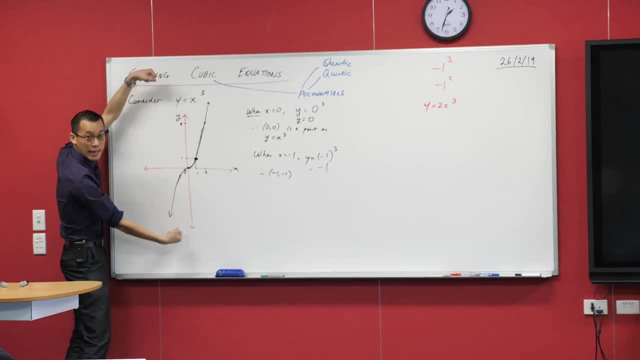 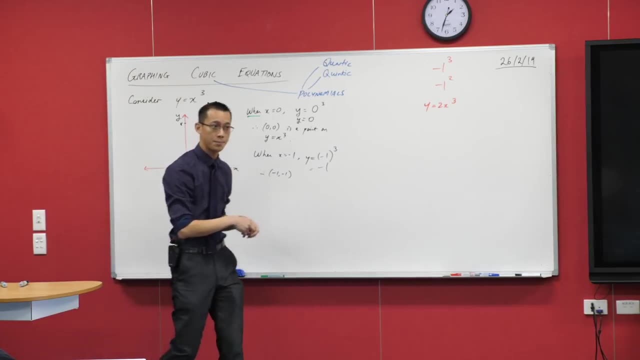 So you're going to get the same kind of shape, but everything is pulled apart like this. It's actually going to stretch vertically or, if you prefer to think about it that way, it's squeezed horizontally. They actually turn out to be the same thing. Okay, Now. 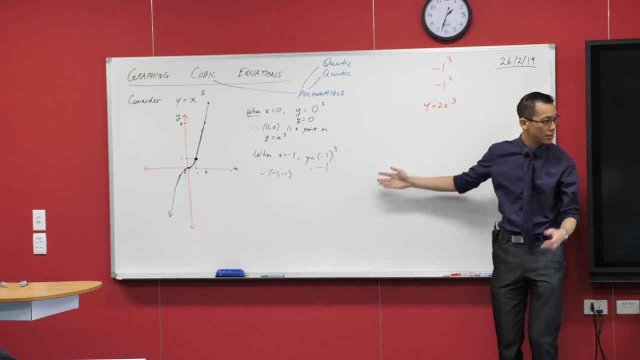 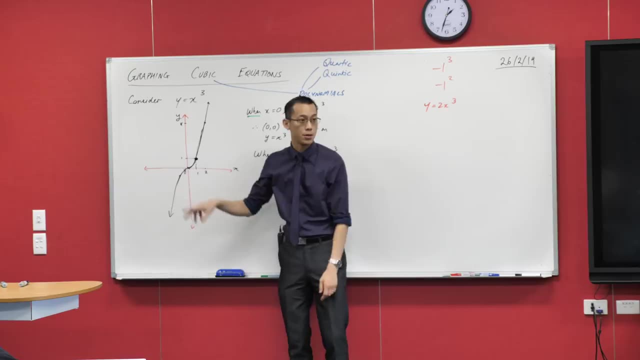 my point is: my point is because they basically have the same shape, but the difference is only scale. you need to provide some kind of information to show you what kind of scale there is. If I took off all of these numbers, you would not be able to tell whether it was y equals. 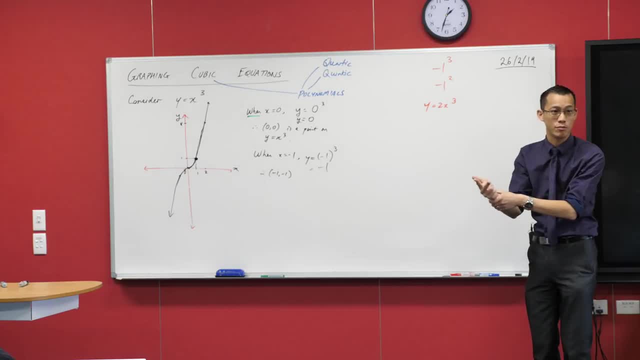 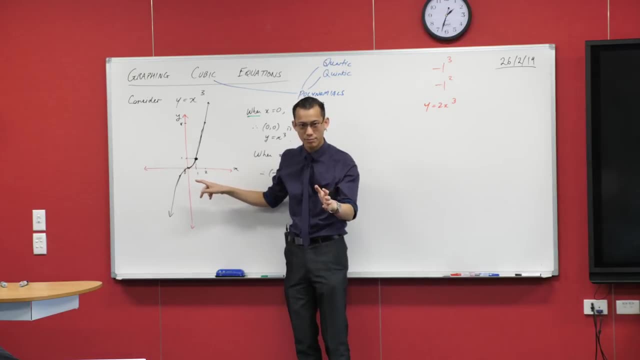 x cubed or 2x cubed or 200x cubed. They all said the same set. Yeah, it's um. these numbers here provide some scale on there. Does that make sense? So an alternative like saying this: saying this is exactly the same, It's equivalent. 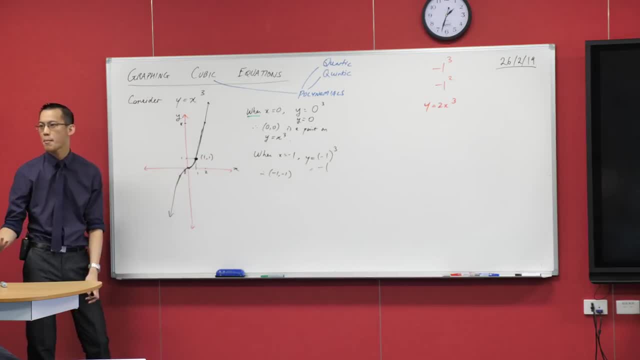 to saying this one comma one: They've got the same amount of information on there, Okay, Um, and you can do either. I don't think you really necessarily need to do both. You can do both because they say the same thing, but you should do one of them, Okay, But because that indicates where that is. Does that make sense? 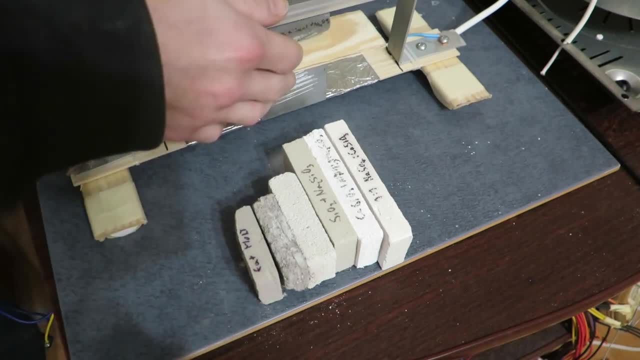 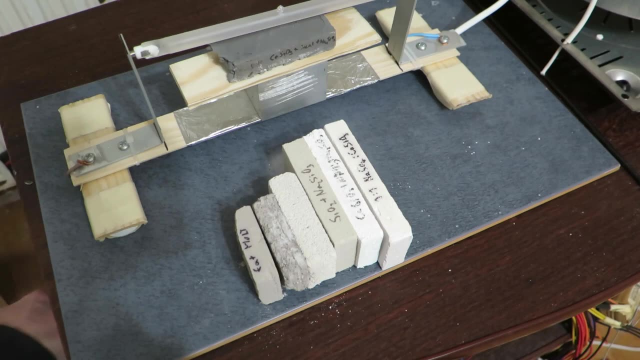 Hi, in this video I will compare thermal conductivity of some fire bricks that I have made. But first of all, this is my setup. I'm using infrared heating element as a heat source. It is transferred by radiation to test subject and it is sunk through a wooden resistor. let's call. 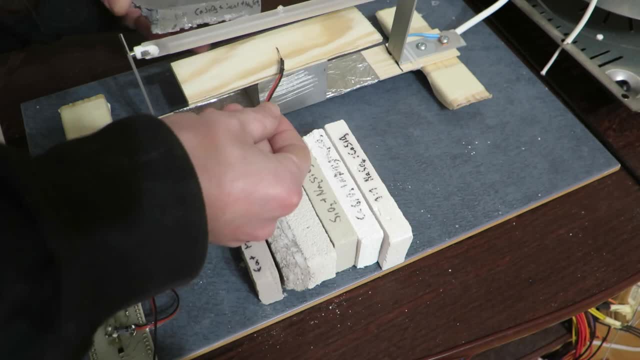 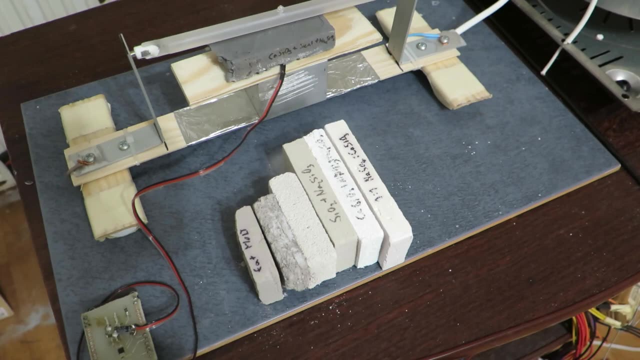 it to aluminium brick and finally to ambient air. This setup is not really perfect, but all I want is consistency during these few measurements, so should be pretty good for that. My goal is to develop material that has very similar thermal conductivity to lining of ceramic hot plate. 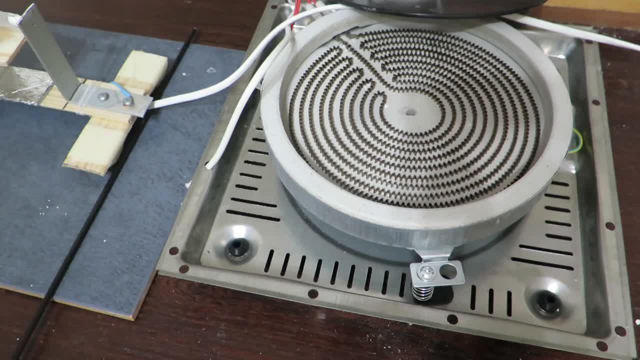 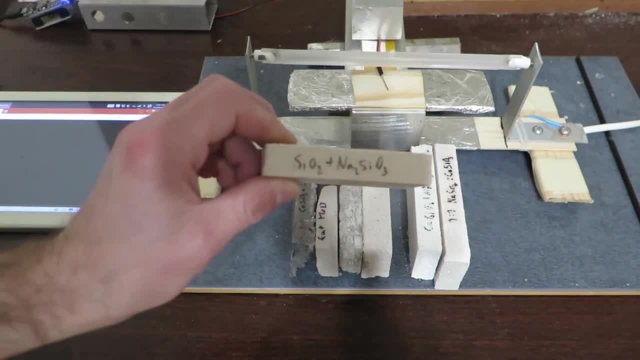 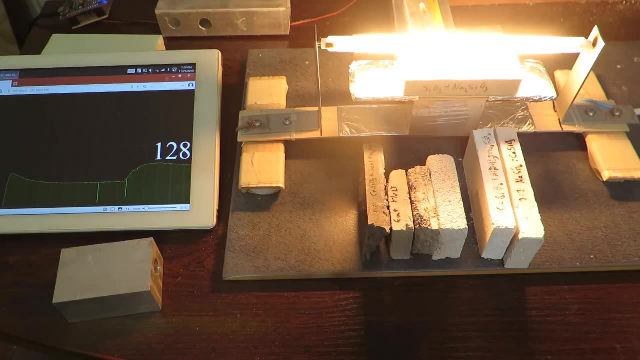 heating element. However, I want it to be castable and with better mechanical stability. Ok, so let's start with this block of sand fused with sodium silicate. After I start heating, I will wait for temperature to stabilize. Here I found out that when the 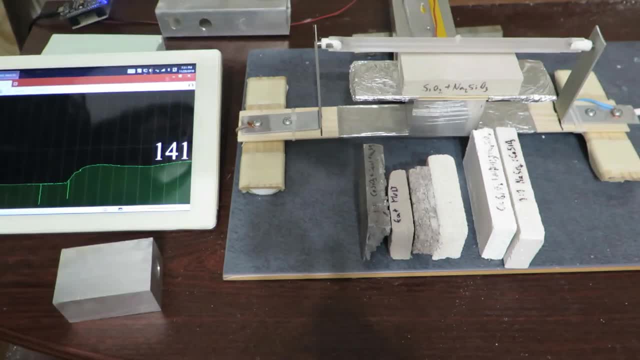 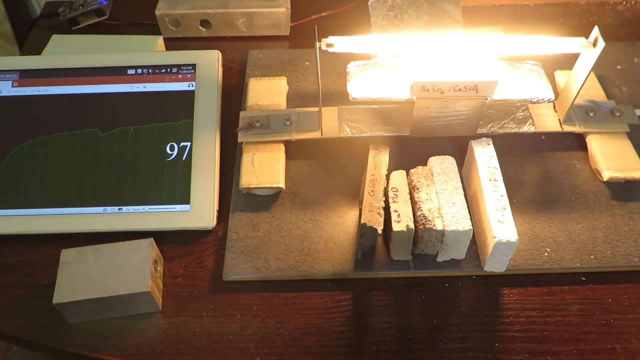 thermocouple lid is hot, temperature reading is lower, so in the next test I will insulate the probe wire. This one is gypsum mixed with calcium silicate. I've got gypsum formula wrong there, so It is not very suitable for high temperatures, but the results are interesting nonetheless.